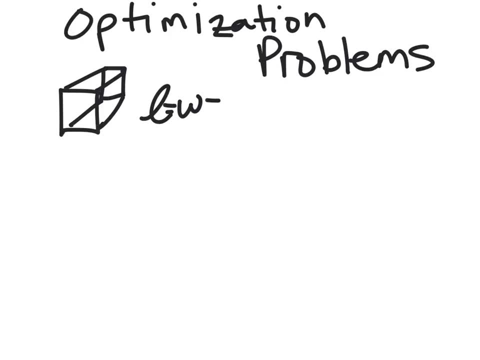 the optimal shape is when length equals width equals height. Remember when we had the really long and narrow 1 by 1,000 snake out in the hall. This is obviously not 1 by 1,000. And then we folded it back on itself and it got a little smaller, And then we folded it back on itself. 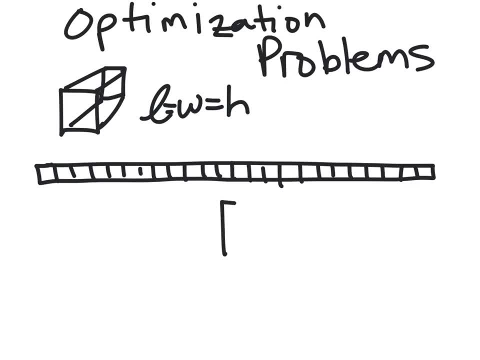 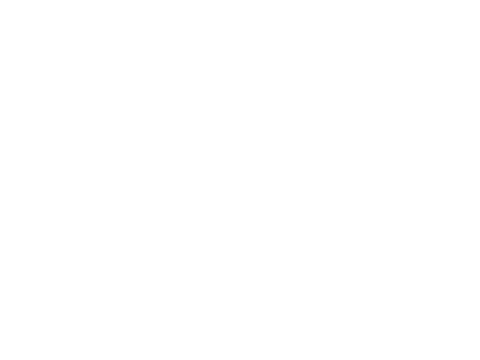 and it got a little smaller And we kept folding it back on itself until that 1,000 centimeter cube volume fit. So what happens if I don't have a cube? What happens if I have a cylinder, Which, as we know, 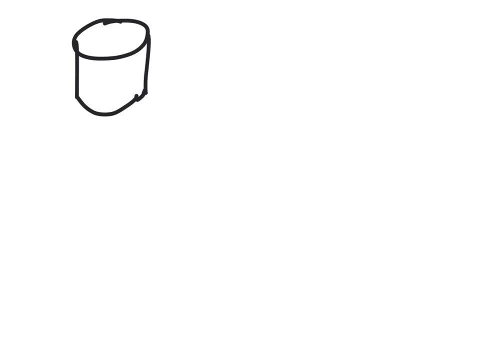 is a common optimization question: What is the optimal height of my cylinder, or what are the optimal dimensions of my cylinder for me to minimize surface area, Looking to minimize surface area While maximizing my volume, Or in other words, what is the smallest surface area I can pack my? 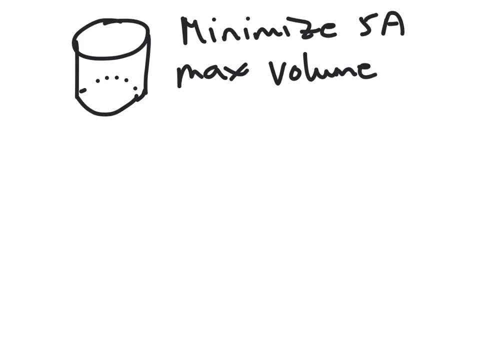 volume into. So of course, I need to look at what dimensions need to be equal. Well, if we think of a cylinder like a cube, it means that height and width right, Because we don't really have a length and a width. 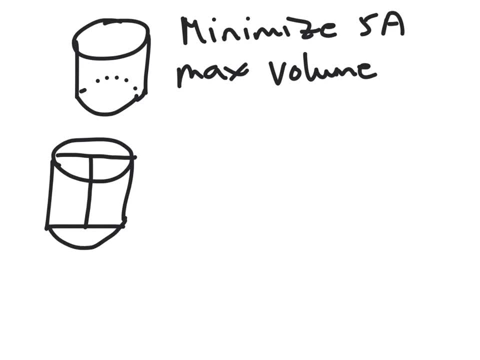 In a cylinder because we have a diameter. So our diameter needs to be the same as the height in order for this to be as cube-like as possible. But when we look at our equations, we don't use diameter, we use radius. Well, diameter is the same as two times the. 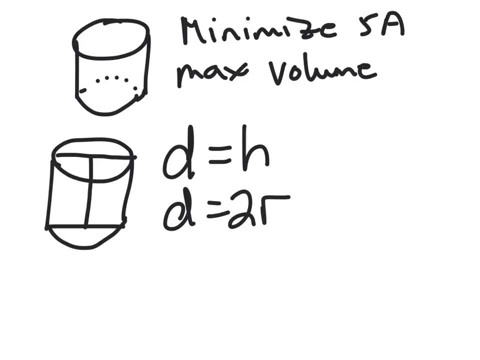 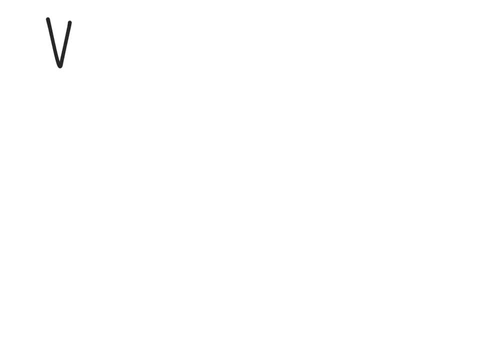 radius. So for my cylinder to have an optimized shape I need my height to equal twice the radius. So let's say I have a cylinder with a volume of, let's say, 2,000 centimeters cubed And I want to know what is the optimum size of a cylinder that will fit 2,000 centimeters cubed of. 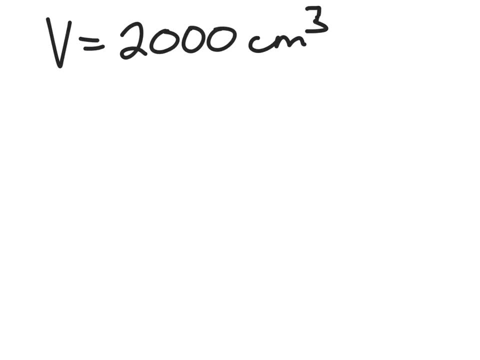 volume. I want to know. so remember to optimize my surface area. it means I'm looking for the smallest surface area for this given volume. The first place I have to start, obviously, is I need to know what my radius is going to be Before I can even think about it. I need to know what my radius is going to be. 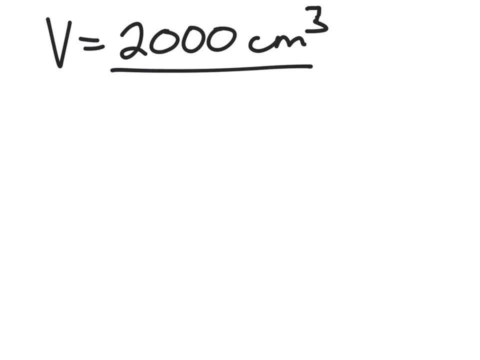 So, because the volume and surface area both involve radius, remembering that my height is going to equal twice my radius- I'm going to have to have the same dimensions for my volume as I am for my surface area. Well, the formula for volume is pi r squared h. So when I'm looking at optimizing this formula, I can say the same as the volume is going to be equal to pi r squared h. 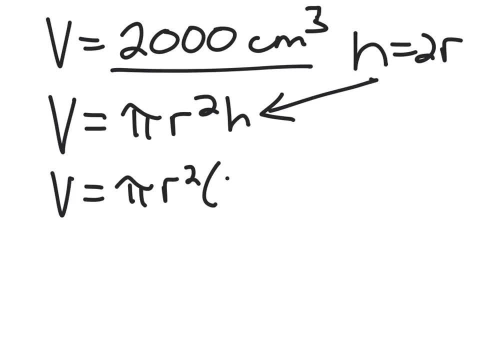 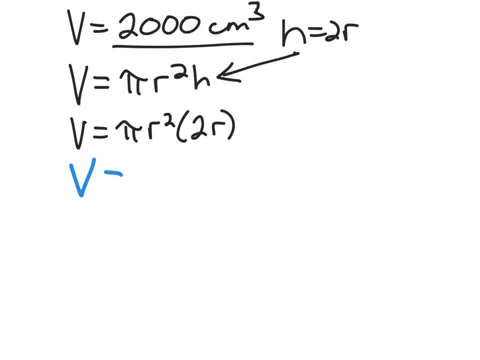 And I'm going to replace or substitute 2r in for my height. Now I'm going to resolve my equation with the 2r for height, So I'm going to multiply the 2r by the pi r squared and I'll end up with 2 times pi times r cubed. That's basically just collecting my like terms. Now that I have done that, I can now rearrange my formula so that 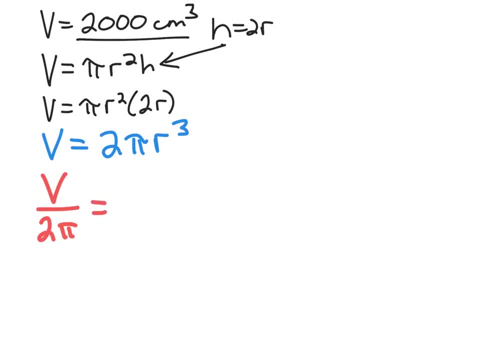 I can solve for r And of course I have to divide both sides by 2pi to isolate the r. And now I'm going to say r is equal to, and I have to take the cube root of r in order to get only 1r. So I have to do the same thing to both sides. So now I have the cube root of volume divided by 2pi. Well, now I have something I can solve. So I'm going to substitute volume for my 2000 centimeters. 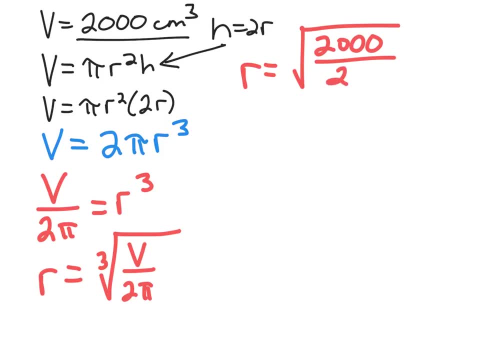 cube that I had in my original question. So I'm going to have 2000 divided by 2pi, which is going to give me a radius of- not quite a radius yet because I still have to take the cube root, but I'm going to end up with 318.5.. And so when I take the cube root of that, I get a radius of 6.8 centimeters. I can now use this radius in a surface area of